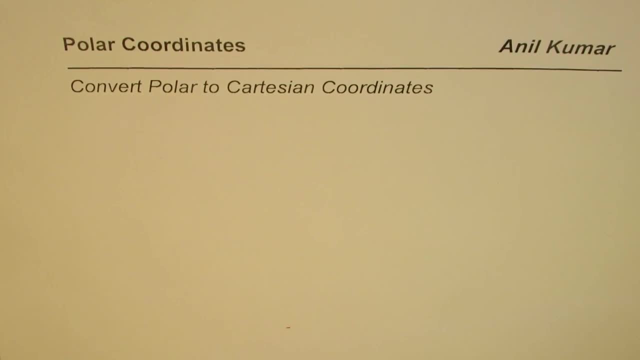 I'm Anil Kumar and in this video we'll understand the basic concept to convert from polar to Cartesian system. Let me sketch our polar system and let me plot a point on it. So in a polar system we do have a pole and the initial arm is the polar axis. So that is what we 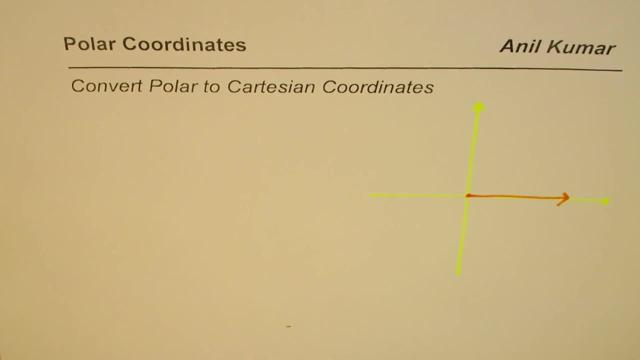 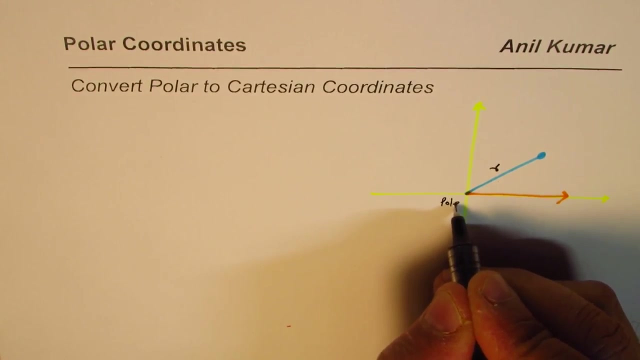 have. Now, if I have a point anywhere, then that point is represented in terms of r and theta. So if I have a point here, let us say, then this point will be represented by two things: The distance from the pole right- this is the pole and that is the polar axis- and 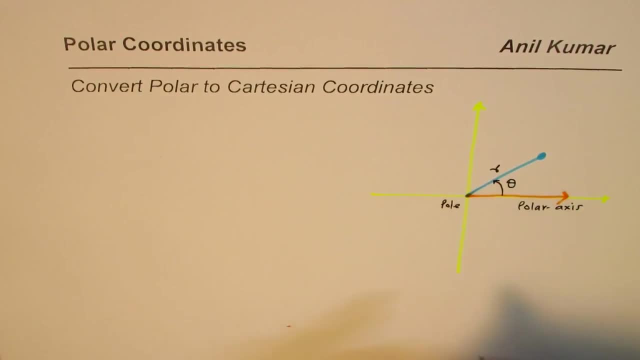 the angle from the polar axis. that is theta. So in general, any point, p will be written as r theta, Is it okay? So we have p written as r theta. Now the question is to convert it to Cartesian plane. When we say Cartesian plane, that means 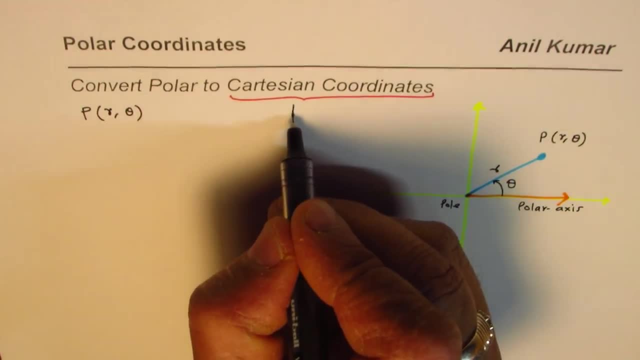 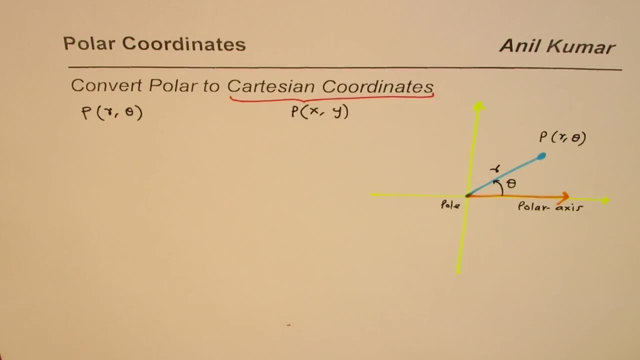 what That means. we are talking about the rectangular coordinate system- x and y, right x and y. So how are they related? The relation is bringing back trigonometry drop of perpendicular. here and now we can say that if we are saying this is a rectangular, 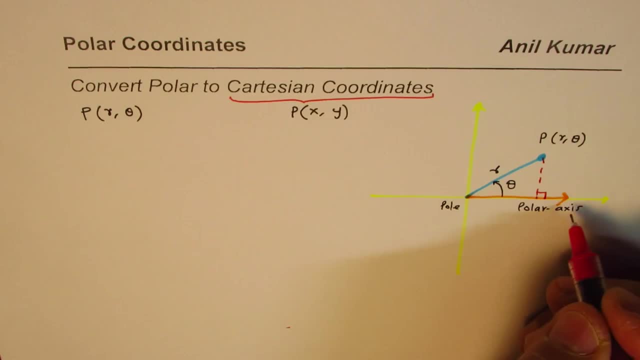 coordinate system. then we will kind of superimpose, We will write this as x and this as y, is that okay? And in that case this distance will be x, right, And this distance will be y. Now, since that is right angle, we can always write relation between x, y and r. 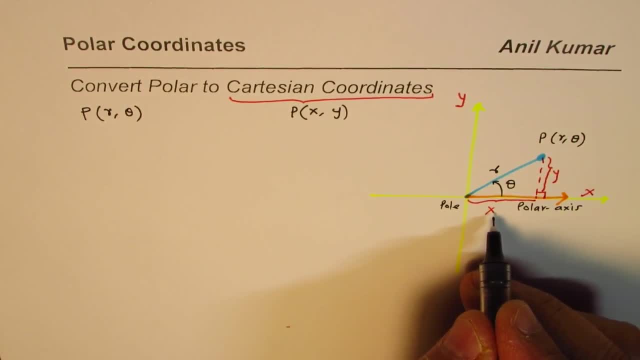 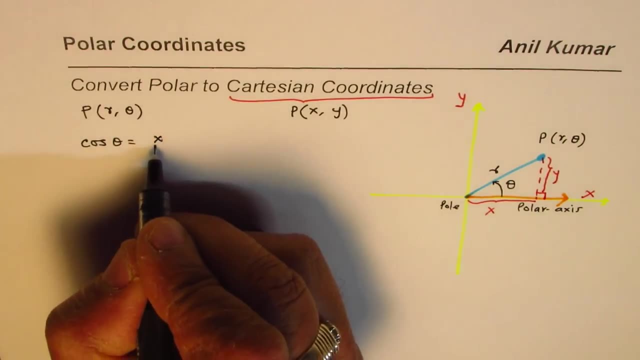 So now, from trigonometry point of view, we know the ratio of x over r is cos theta, right. So cos theta is ratio of x over r, and that gives you the value of x as equals to r times cos theta. 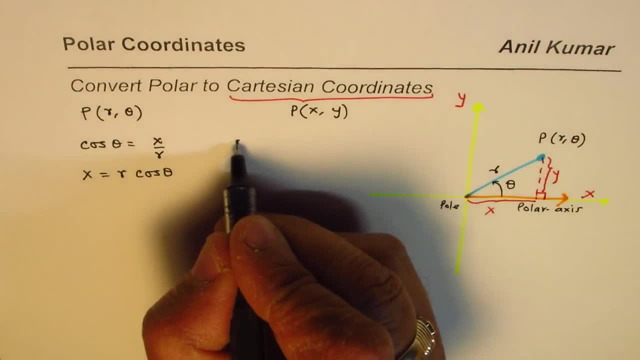 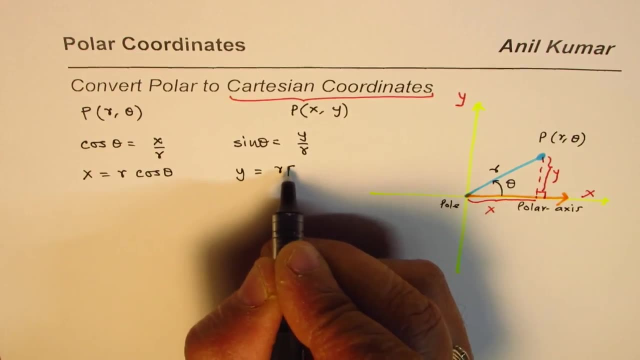 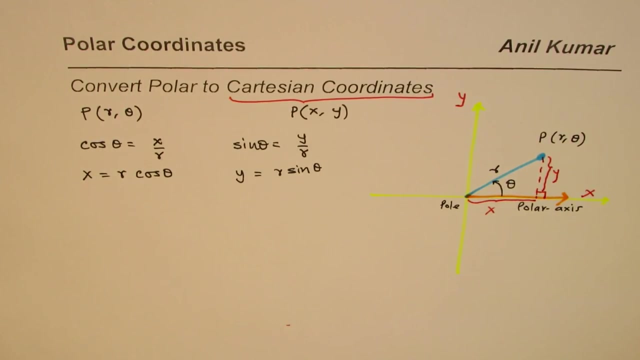 right. As far as the y value is concerned. sin theta is the ratio of y over r, So that gives you y equals to r times. sin theta, sin theta, right, And that really gives you the points x and y correct From the polar coordinates. 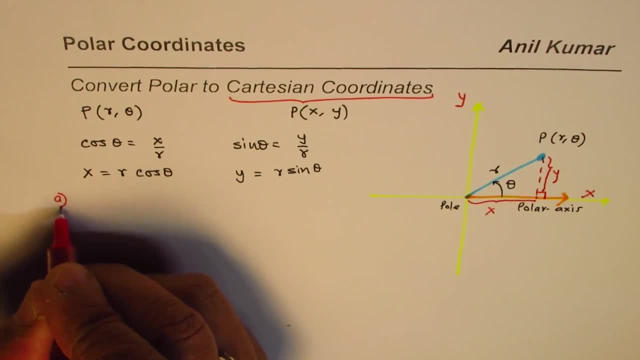 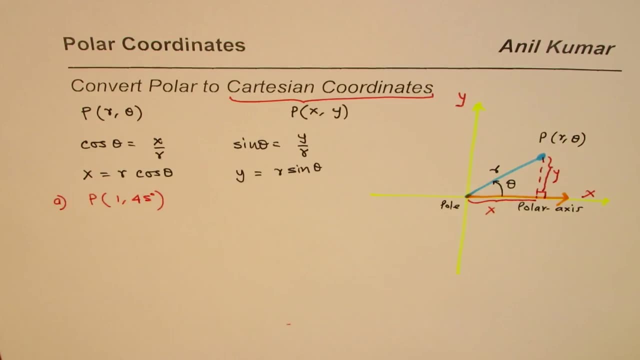 Now let's take a few examples. So example A for us is a polar coordinate. let's say 1 and we'll have 45 degrees to start with, okay? So when I say 1 and 45 degrees, in that case, 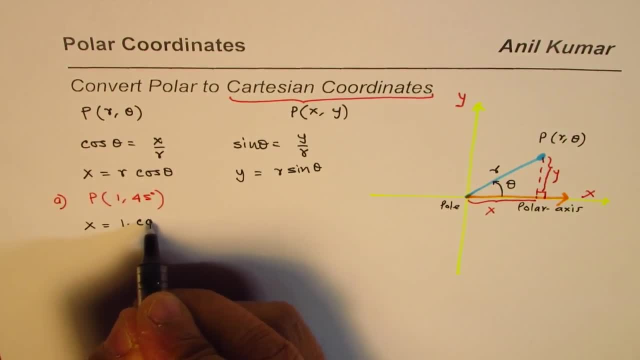 x will be one time cos of 45 degrees, Right, Which is- let me write 1 here, which is 1 over square root 2, or square root 2 over 2, correct. So that is what the point is. and the y value will be one time sin of 45 degrees, and that 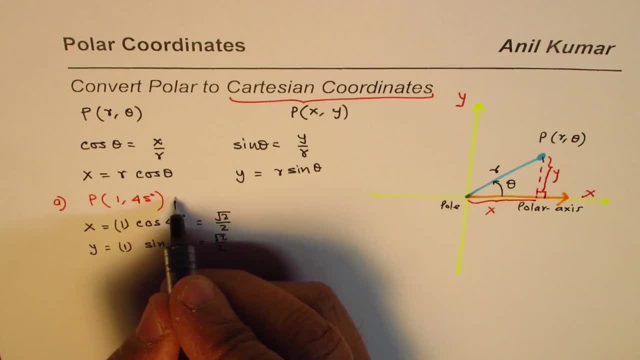 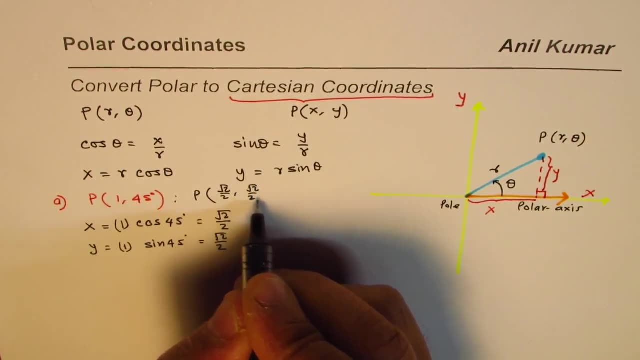 is also square root 2 over 2,, correct? So we do get an equivalent point. which a point could be written as square root 2 over 2? comma? square root 2 over 2, is it okay? So that is how you could. 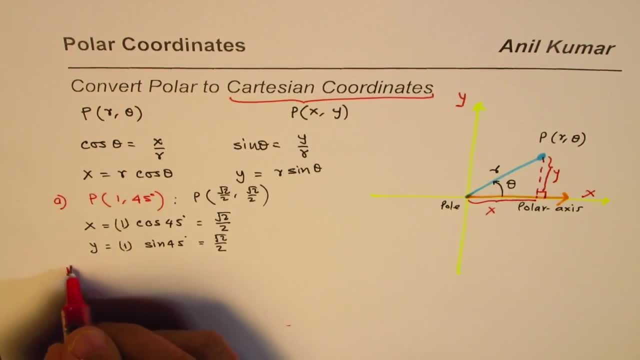 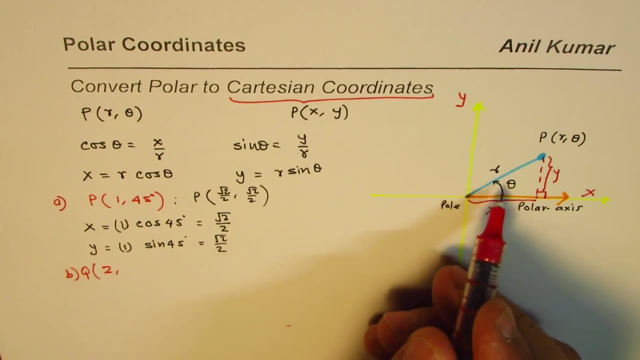 easily write it. Now, if I take another point B and let's say this point is, let's say Q is 2 and the angle is, let us say, 120 degrees. okay, So this time we'll write our point as we could. 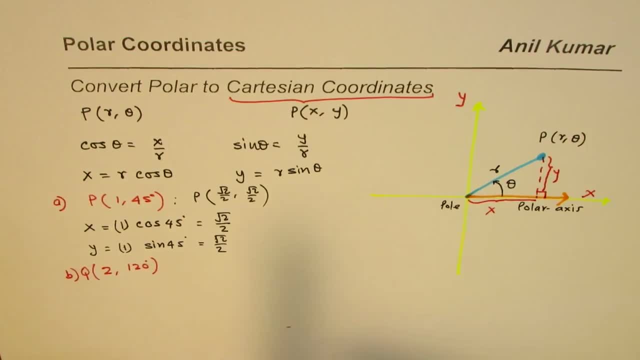 write in decimals or in exact values also. So using the same formula, we can write the x coordinate point as r, which is 2. 2 times sin theta. 2 times this is r and theta right 2 times cos of 120 degrees and the y coordinate point. 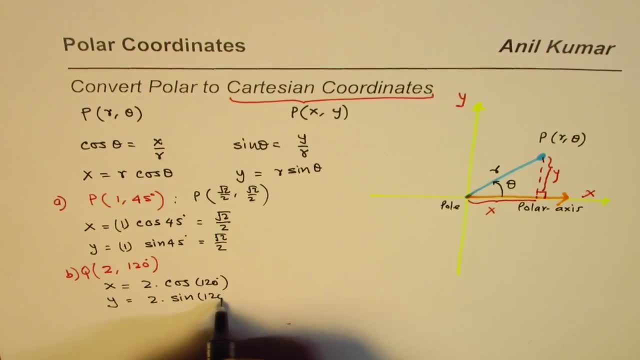 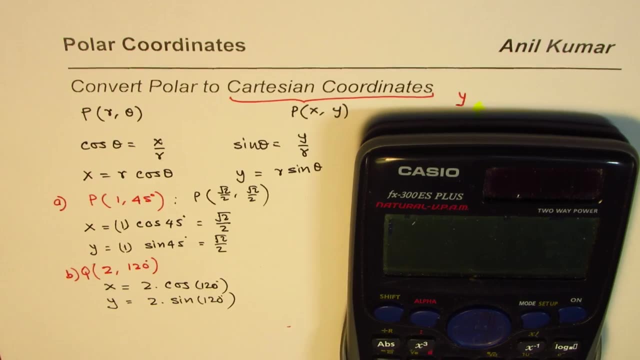 will be 2 times sin of 120 degrees, right? You can use calculator to calculate, right So you can have. you know what is cos of 120 degrees. So it will give you a negative value, right? So it is 2 times. we say cos of 120 degrees equals to negative 1,, right So? 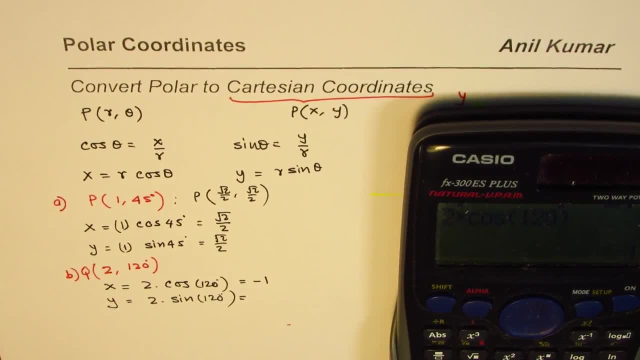 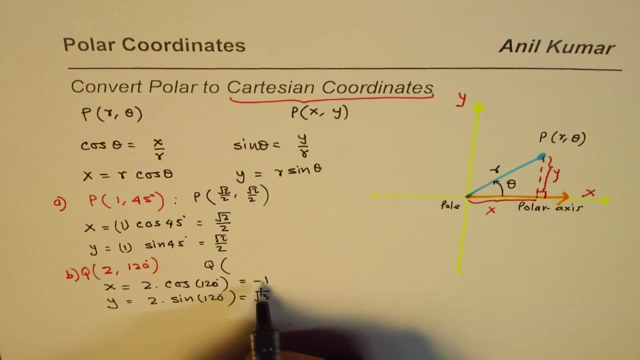 this gives you a value of negative 1,, as far as the y value is concerned, 2 times sin of 120 degrees, and that gives you square root of 3.. So this is square root of 3.. So you write this point Q as the x value is negative 1 and square root of 3, correct? Now let 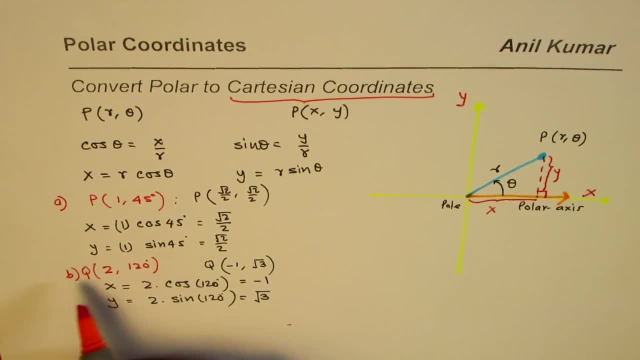 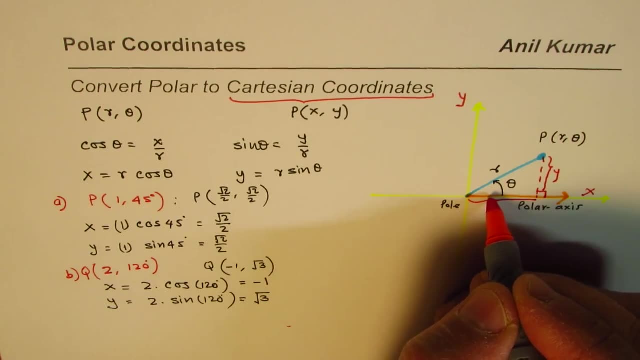 us see if it really confirms to the value here: 2 and 120.. So 120 is the angle, 120 will be kind of this is 90 and 30 more correct. So it is kind of like this: that much is the angle correct And 2 units. So let us say this: 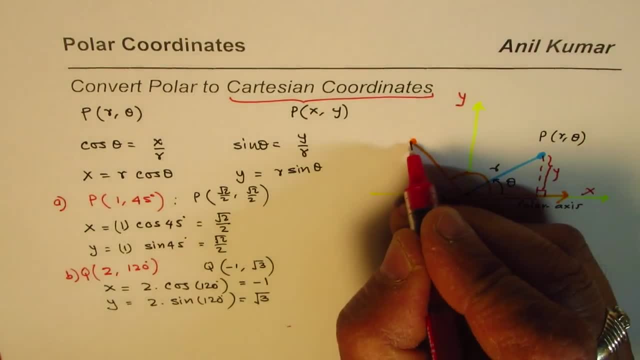 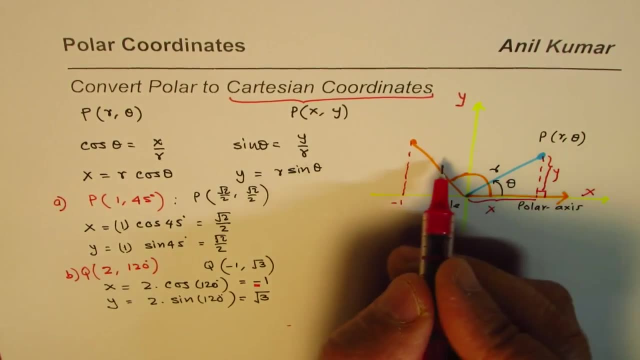 is 2 units for us. So clearly, in this particular case we have x. value is negative, right, So it makes sense. it makes sense, This is 2,, right, And we are saying this. this tends to square root of 3, and that is positive, right. 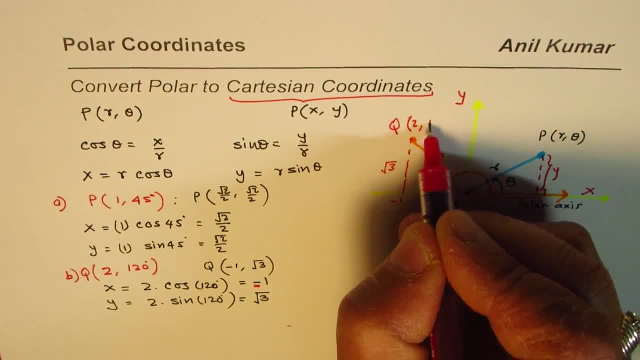 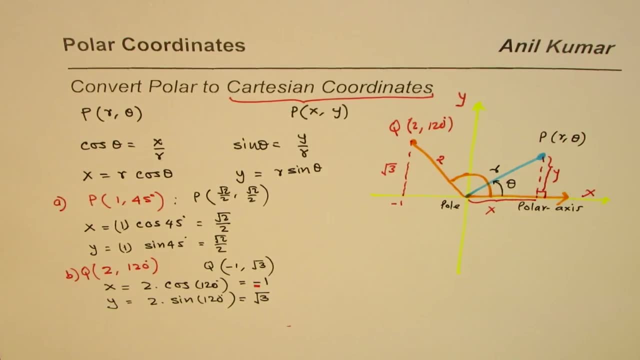 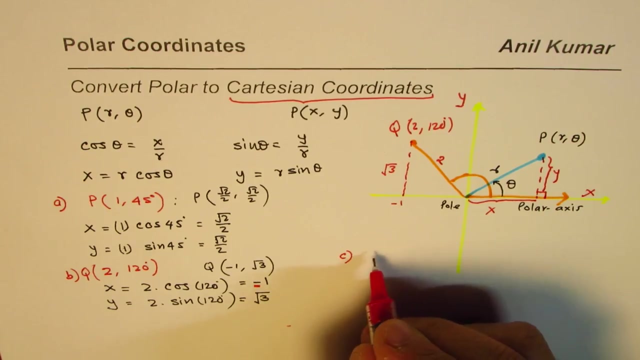 So that is the point Q for us, which is 2, 120 degrees on the polar coordinates. But when you translate it on the Cartesian coordinates, you get that value. Does it make sense to you, right? So we can convert any point, right? Let me take another example here and 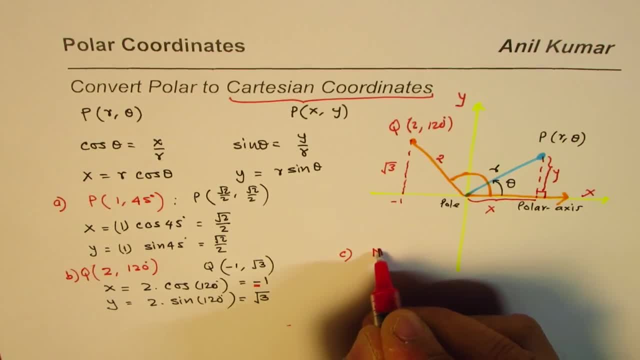 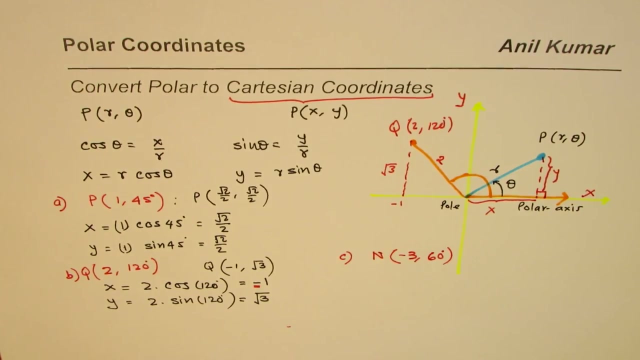 let us say the point is n for us and this point n is minus 3 and the value here is, let us say, 60 degrees, right, Okay, So minus 3, we have taken right. So if the r value is negative, 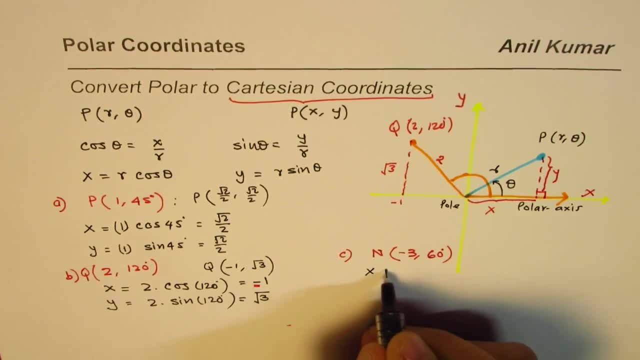 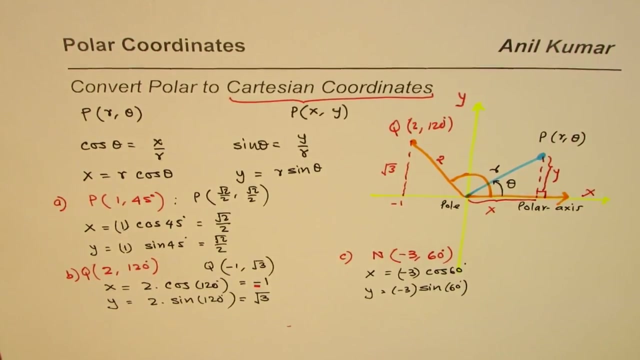 3,. in that case what happens? x value becomes r is negative 3, right? So negative 3 times cos of 60 degrees and the y value will be negative 3 times sin of 60 degrees, correct? Let us use the calculator again. So so we will do negative 3.. So negative. 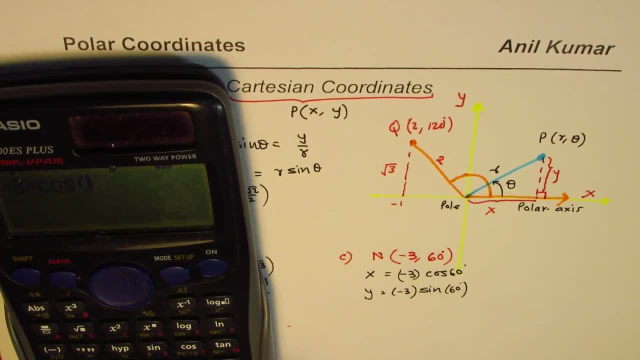 3 times sin of 60 degrees. right, So we will do negative 3 times sin of 60 degrees, right, So that gives us minus 3 over 2,. right, So this gives us minus 3 over 2, and. 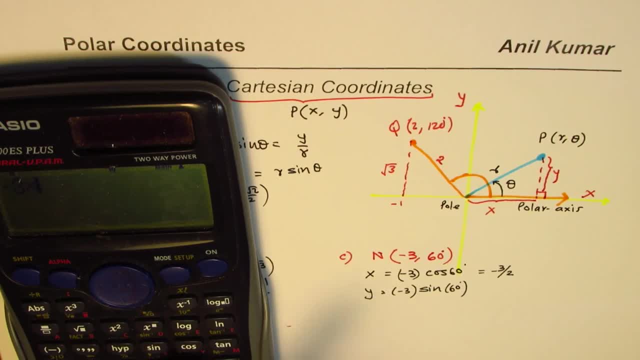 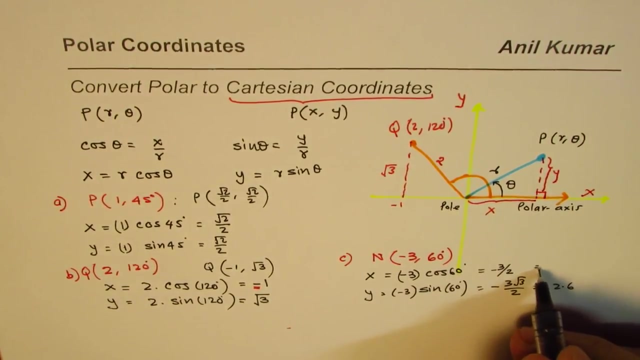 let us do negative 3 times sin of 60 degrees and that gives us minus 3 square root, 3 over 2, okay. So these are the values which we get If you want to convert to decimals, like minus 2.6, approximately, okay, And the other one is minus 1.5.. So this is minus 1.5.. Is. 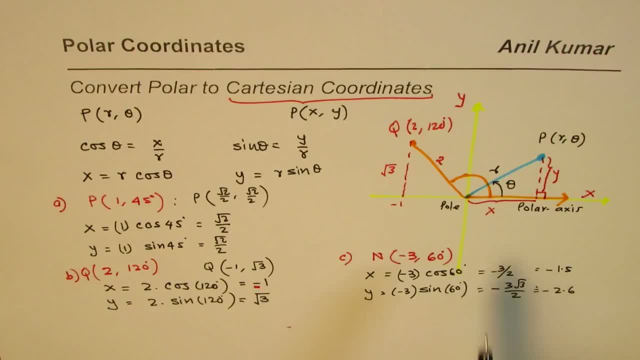 it okay. So we get both negative values here, That is to say, we are trying to see the point n in the quadrant 4.. If it fits for both, right Is it? so? Let us look into it So. 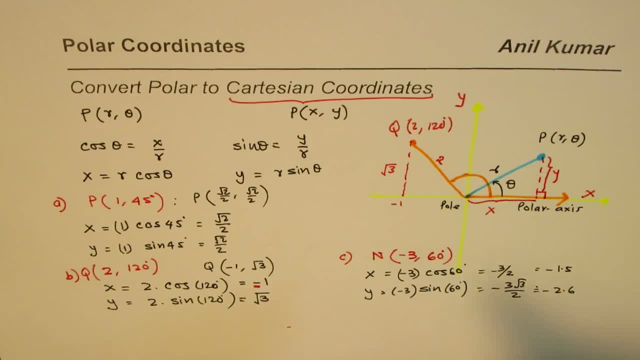 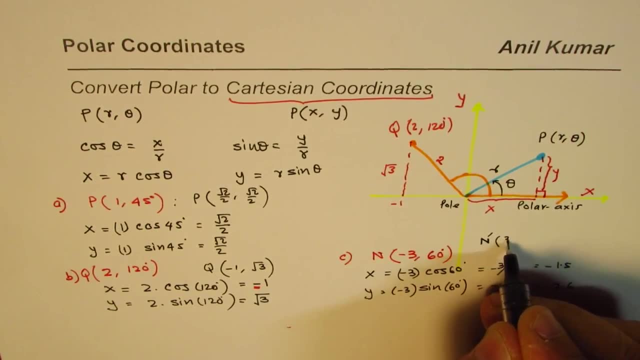 what we will do is we will kind of sketch this. So minus 3, 60. If you have to sketch this, you really sketch the image first, which is 360, right, So 360 degrees. So let us. 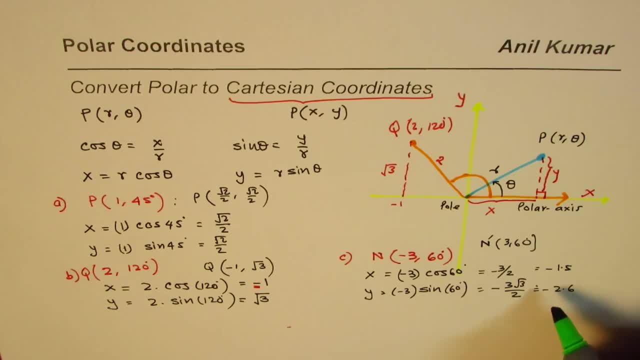 say that the we will use this pen 60 degrees. is this much for us, right? 3 is kind of longer. Let us say this is 3 for us, Okay. So this is the point n dash. So n will be, n will. 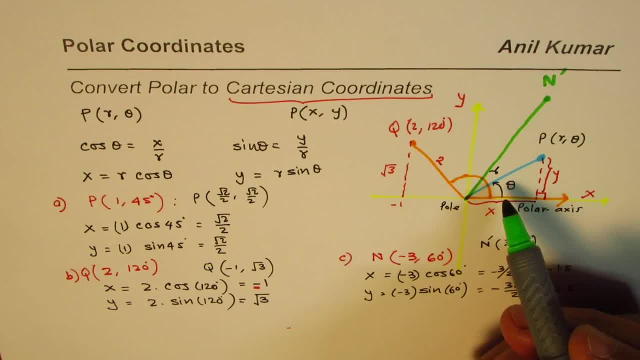 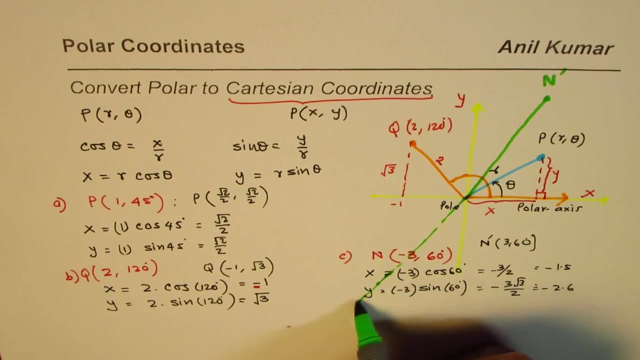 be reflected, Is it okay? So 60 degrees and 360.. So it is going to be reflected here. So when you reflect this, you get a point here. Okay, Let me sketch this. Let us say: this is the point, right. So that is where we get. 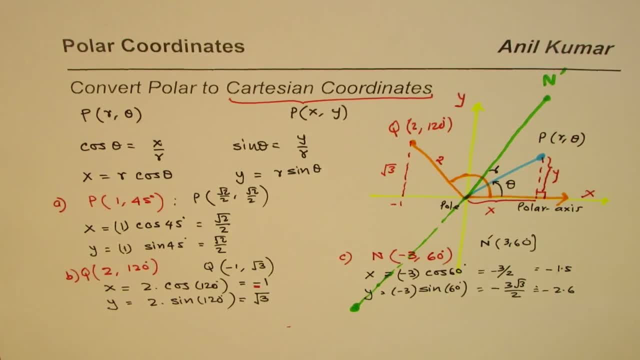 our point Now. minus of 30 and 60 degrees is a point here. Now, how do we relate this to the result? The result is showing that both are negative, Correct. So since both are negative, you can very clearly see this is minus. this is the point n right. So this is the point. 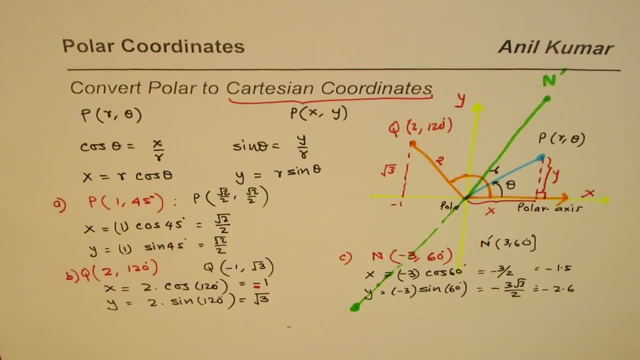 n. Let me use another ink now. Okay, So this is the point n. Let me push it a bit, Okay. Okay, So this is the point n. Let me push it a bit. Okay, Come on, I am going to let it just. 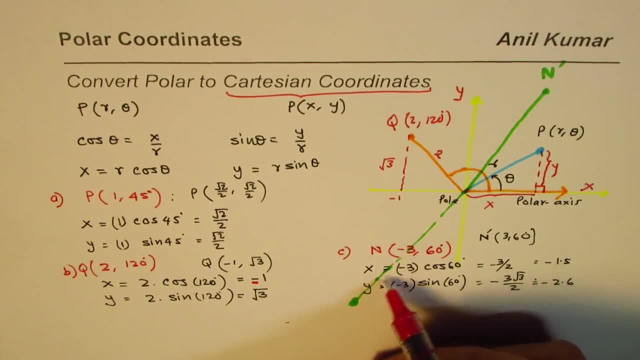 reflect it, The whole thing. I made it a bit longer. I did not want to write in between here and mess this up. Okay, So we get a point n here which is minus 360 degrees, and well, this sketches not to the scale, So anyway. so what we get here is a point which 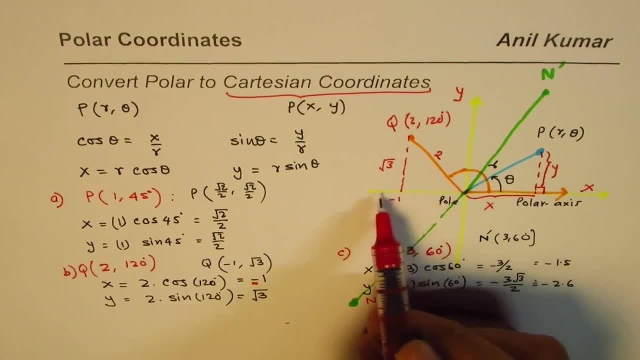 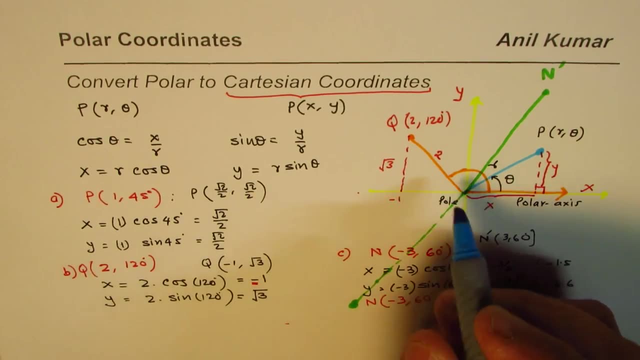 has x value of minus 1.5.. Does it make sense if you see, right, Okay, Let me kind of use another ink here just to highlight this portion- what we see here is that the x value if you look into the coordinate plane, right? so what you get? 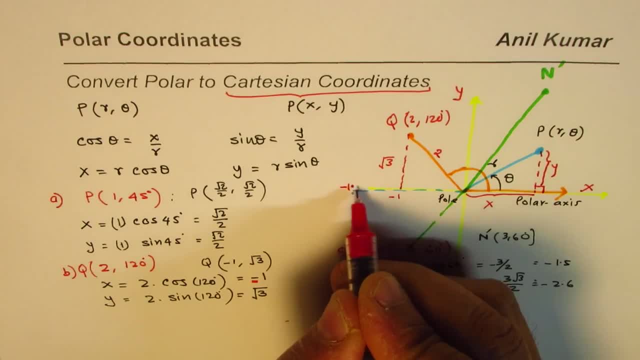 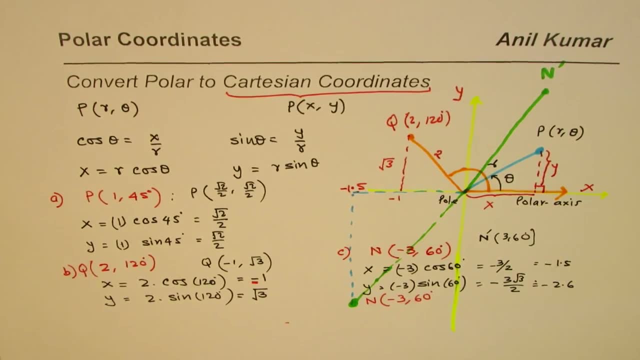 is kind of like this. so let's say: this is a minus 1.5, is it okay? and the y value: okay. let me sketch this, i didn't want to spoil that. okay, anyway. so this is my y value, which is minus 2.6. let's say: 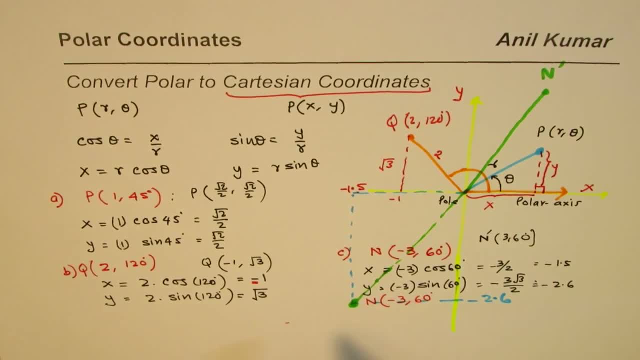 right, so you get an idea. so that point here is n, so it fits very well with the concept we have learned about. polar coordinates and cartesian coordinates fits in right. so so a negative point, i mean the negative distance, r could be represented like this and you have its equivalent on the. 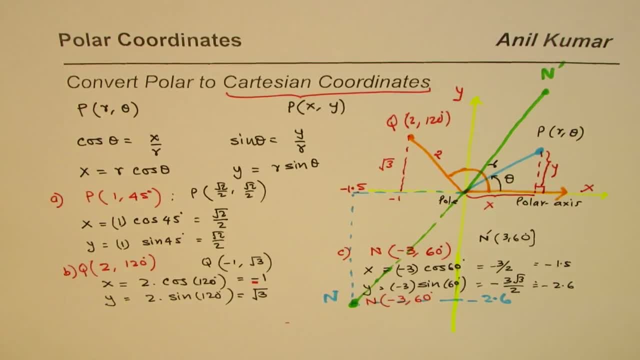 cartesian coordinate system, as we just saw it right, amandil kumar, and i hope that helps you to understand you how to convert from polar coordinates to cartesian coordinates and also how to sketch them right. so we're kind of superimposing two coordinate systems one over the other in this case. 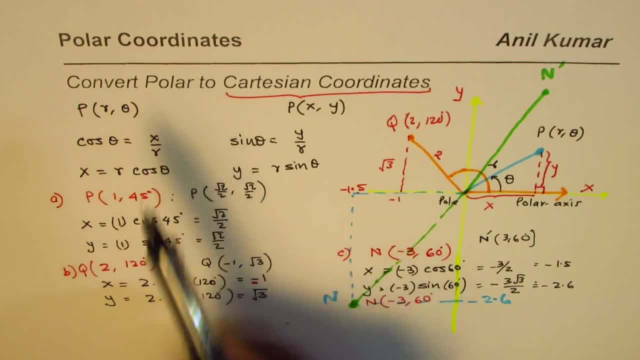 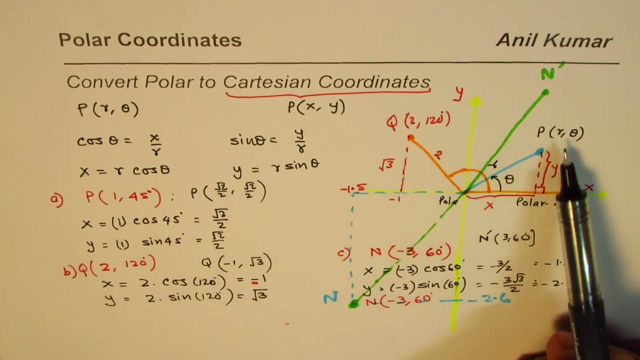 so don't really get confused. when we talk about polar coordinates, we are only looking to the pole and this axis, but when we talk about cartesian, we're looking into x and y, correct? so these values which i've written here in numbers, they relate to the cartesian coordinate systems. when i'm 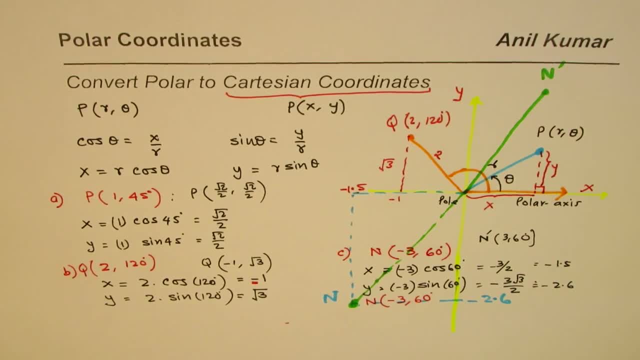 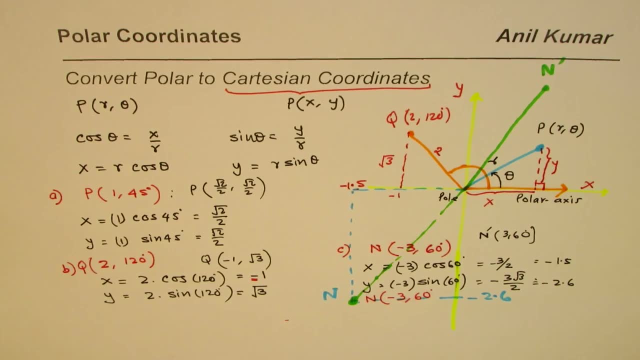 writing r and theta. they are for polar coordinate systems. i hope that makes sense. amandil kumar, you can always share and subscribe my videos. thank you and all the best.